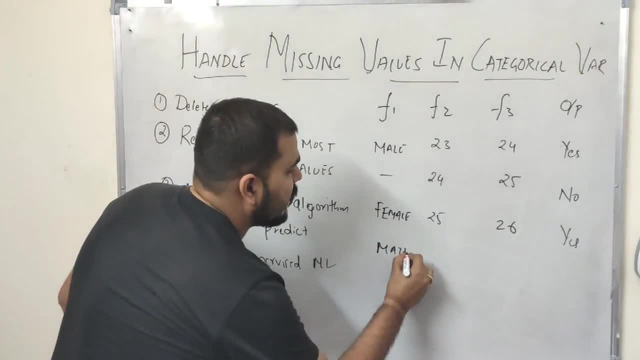 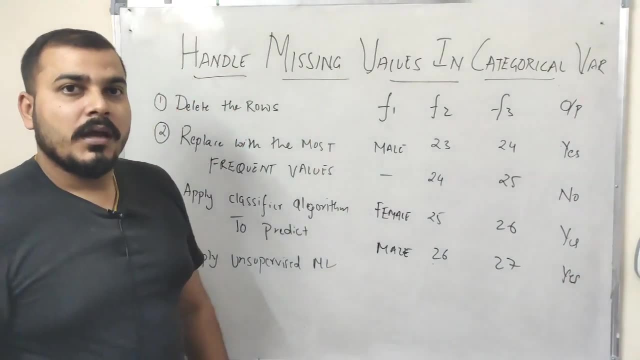 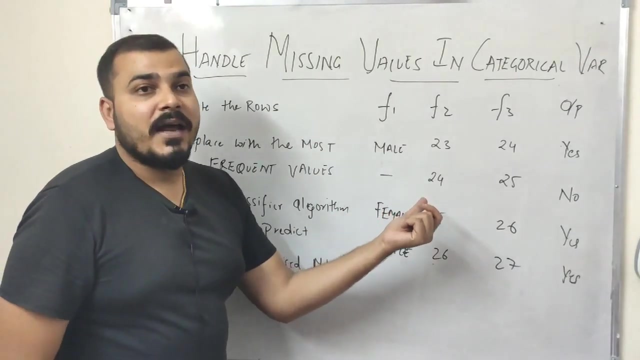 I may have still male again. I may have some records over here and again I may have the output variable And similarly like this. it will continue Now over here. you observe that I have some missing values over here. So what are the various different ways we can handle these missing values in a categorical feature that we are going to discuss? 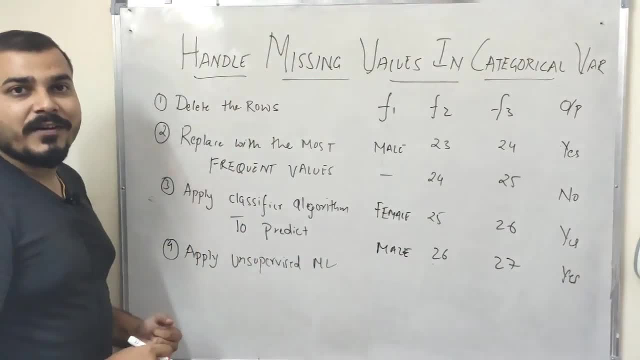 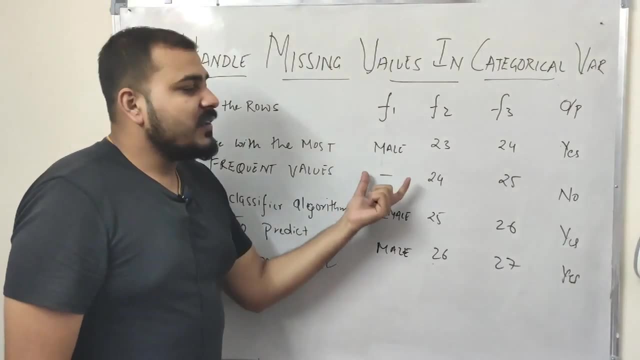 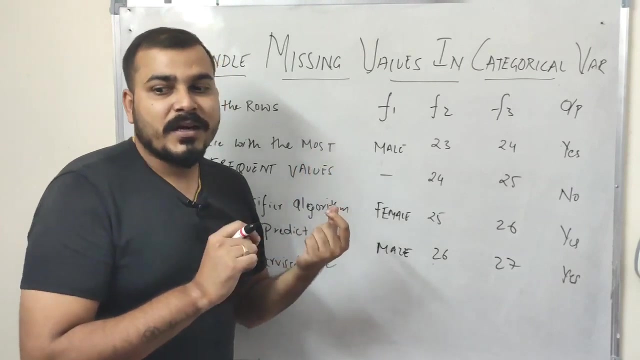 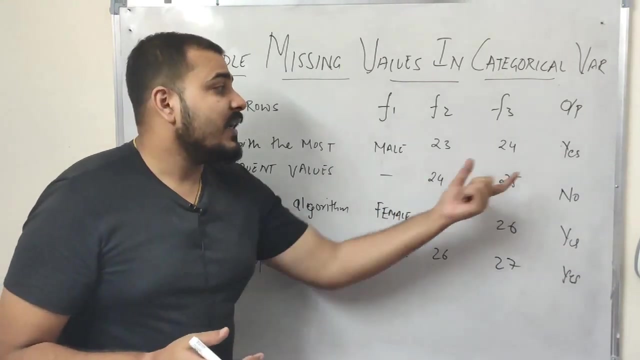 So the first: I have basically noted down all the different ways how you can handle it. The first technique is basically deleting the rows. Now, wherever this particular empty cell is basically present, what we can do is that we can delete the complete row. But remember, guys, if we follow this particular step, it may happen in such a way that this data set, or the records that I may be deleting, may be important for my classification problem. 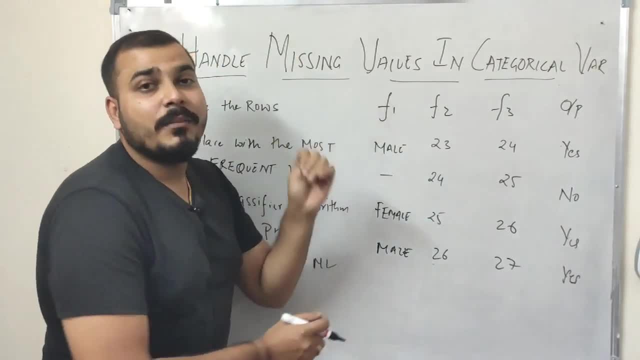 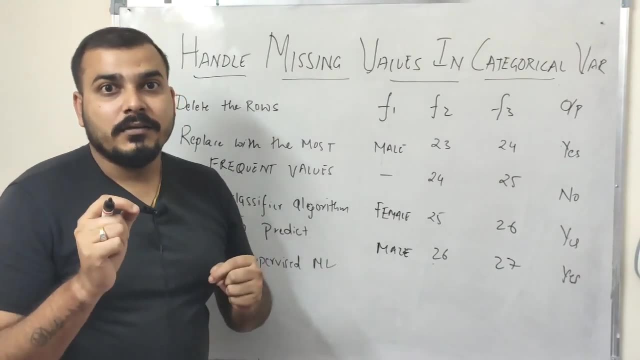 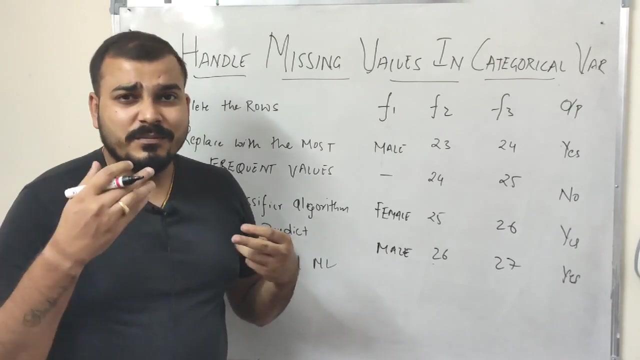 And I cannot delete the rows if I have a smaller number of data set, when my number of records are very, very less. So there is a lot of disadvantage for that. So never go ahead with that, Never delete the records. Now if suppose, if you have million of records and in that suppose you have 2 to 3 of very less number of records where you are having missing values, then you can basically delete it. 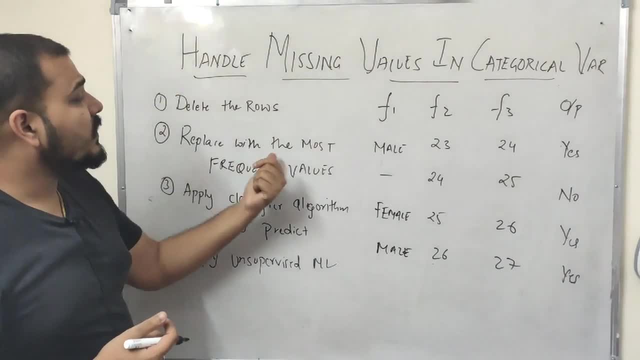 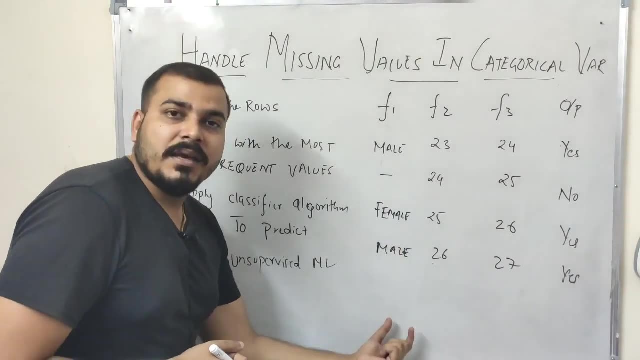 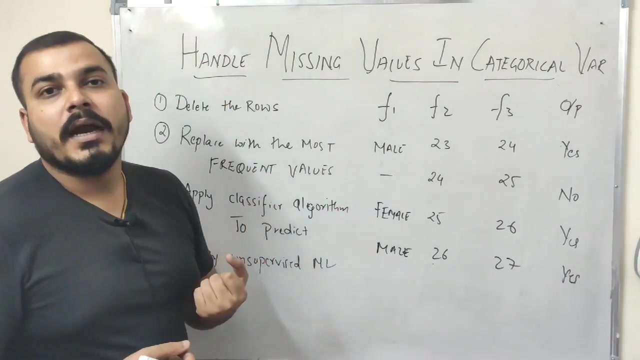 Now the second method is basically replace with the most frequent values. Now suppose in this particular data set, suppose I had most of the time female coming as the categories over here. Now what I can do is that I can replace all the missing values with the most frequent occurring category. 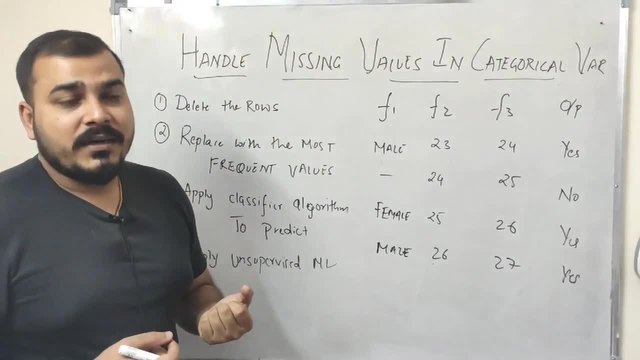 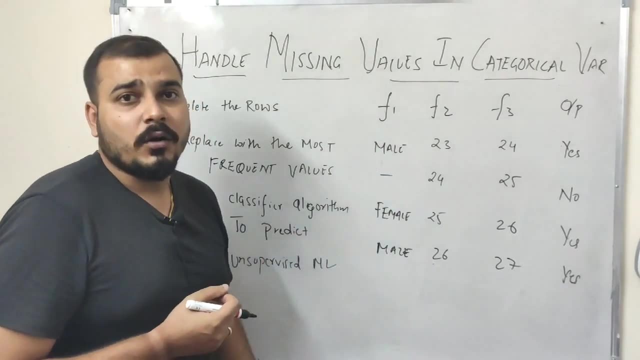 So that is basically the second technique. Okay, But this may also lead to some one kind of problem that is, imbalance data set. Okay, Now suppose I have, suppose, thousand record over here, and suppose 700 records I have female and 200 records I have male. 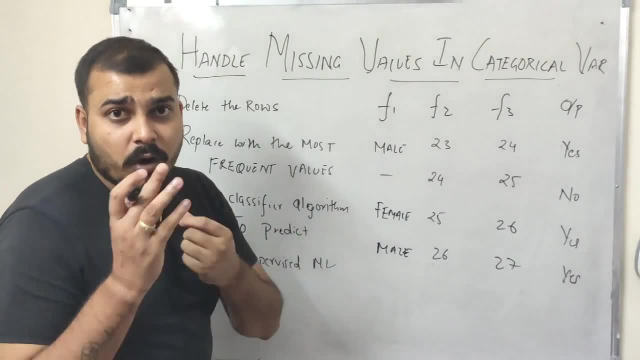 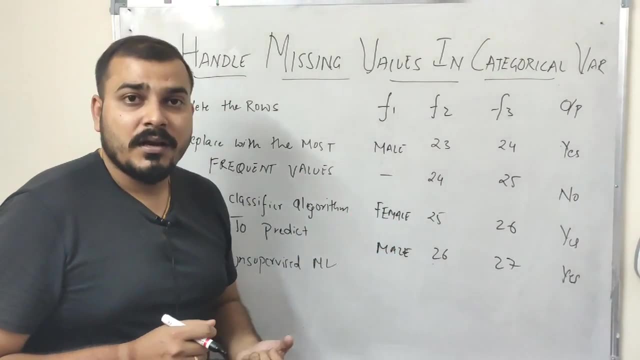 Right, And then the missing values. according to that condition, what will happen? that will try to replace with the most frequent values, and the most frequent values in this case is basically female, So it will become 700 is to 300, right, 200, sorry, 800 is to 200. 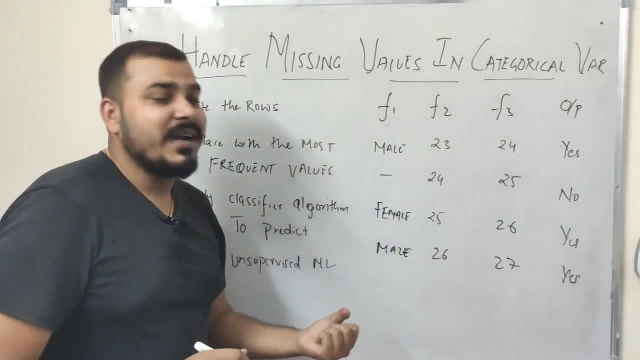 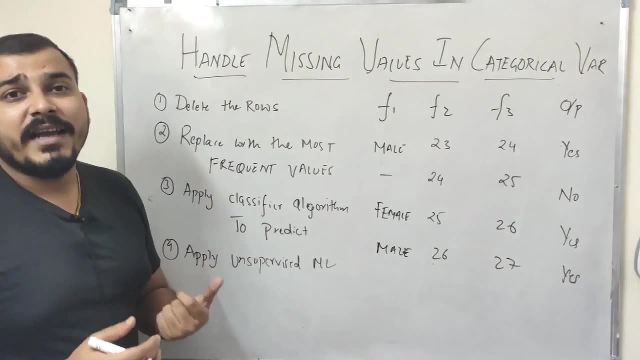 So again, that will lead to some kind of imbalance: data set within the categories, not with respect to the output variables. Okay, Now the third technique is basically the most efficient technique. You create and classify algorithm to predict this particular category. Now how this will work. 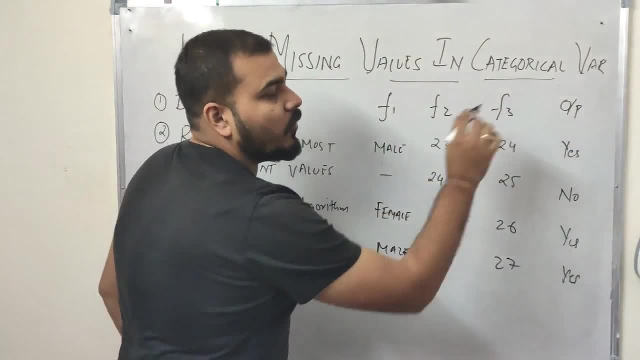 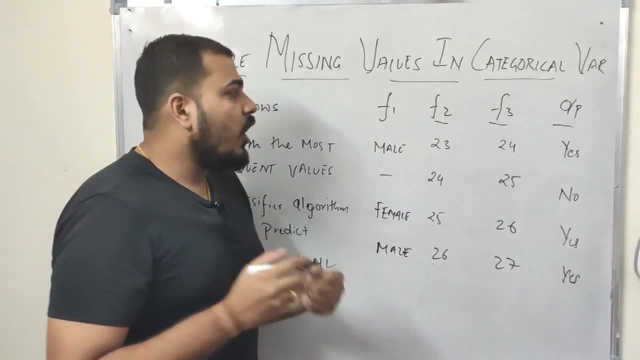 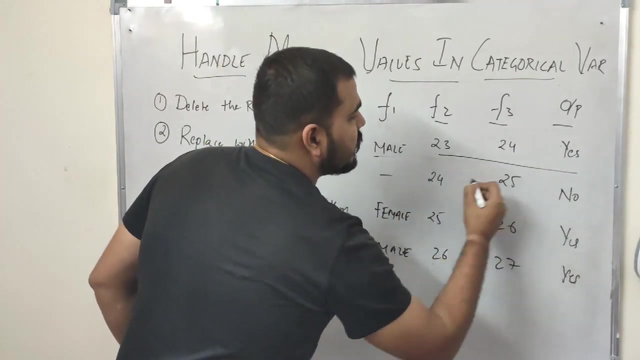 What you have to do is that I have my feature F1, F2, F3 and output. What I will do: I will make F2, F3 and output as my independent feature. All my training data set will be this record. Sorry, all my training data set will be this record. 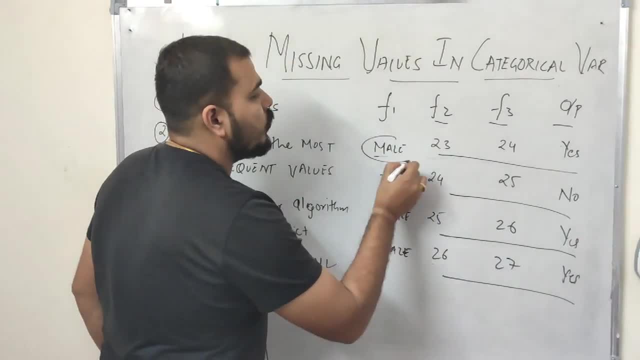 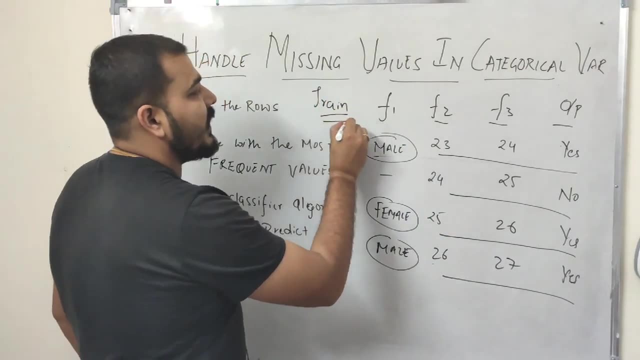 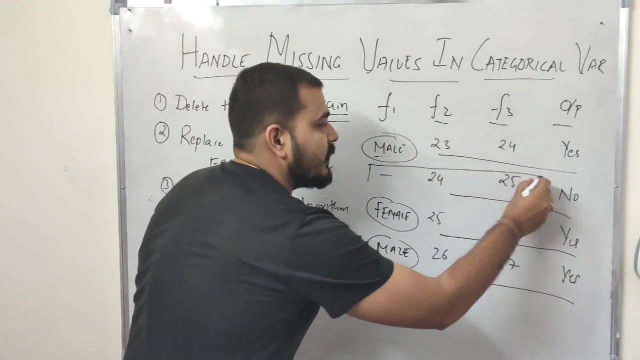 Okay, And wherever I am having this output value, I will consider all this as my train data set, As my train data set. Okay, And wherever I have this blank values, that will basically become my test data set, Because in this training data set, what I will do is that I will consider this as my output feature. 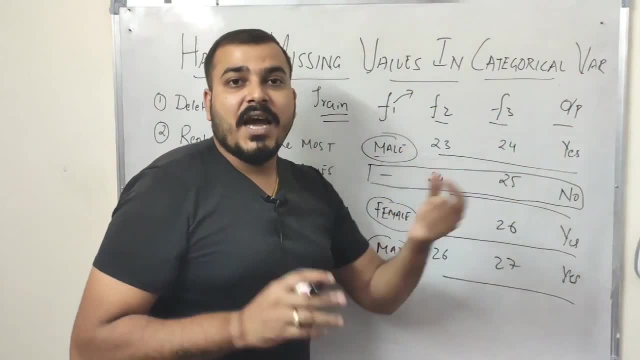 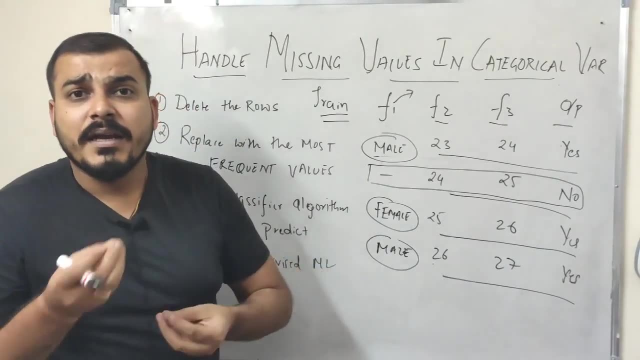 Taking this as my independent feature, I will create a model And it may be a classifier model right Based on the number of categories. It may be a binary classifier. It may be multi, multi categorical classifier. It depends on the number of categories present in this particular value. 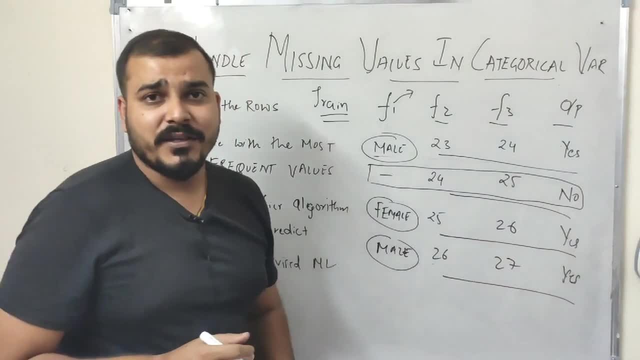 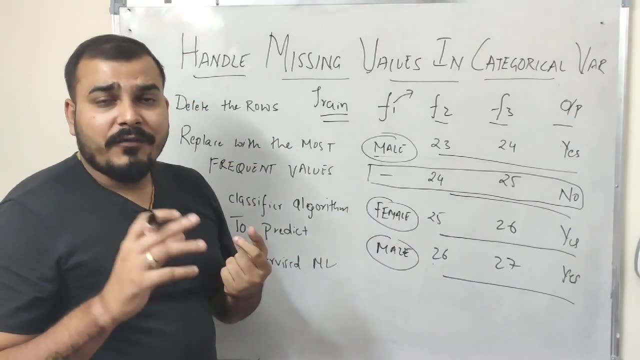 Okay, So in this case, what I will do is that I will take this as my independent feature. Use this data set for training my model, which will predict the output that is my F1.. Now, after my model is trained, I will take all this training data set. 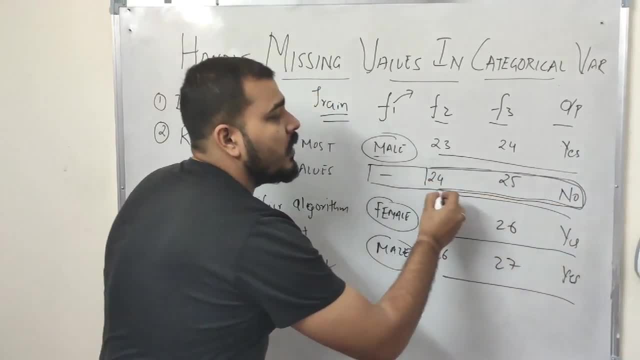 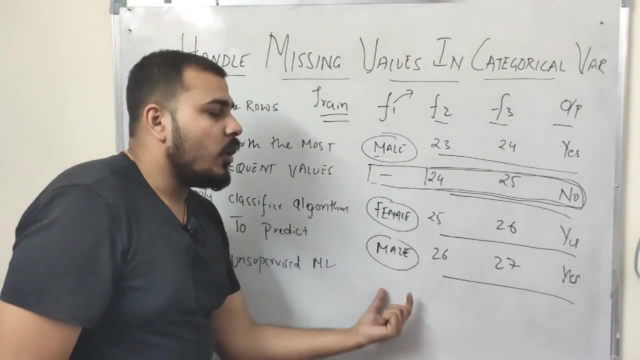 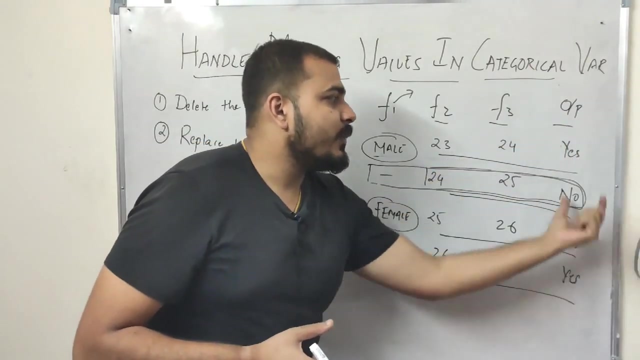 Only give my this independent feature record. My model will then predict what will be the category for this particular value And once we get the category, I will start filling all the empty values with this And later on what I can do is that I can basically create my own machine learning algorithm finally, to predict the output column. 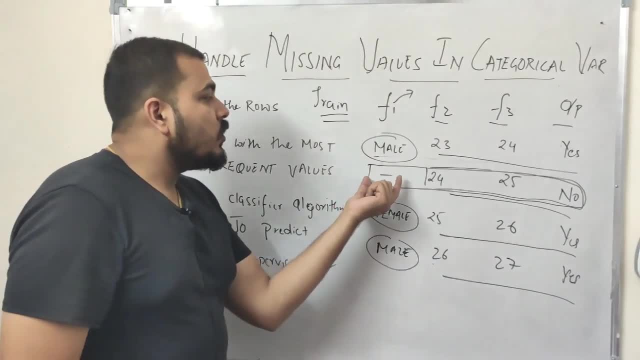 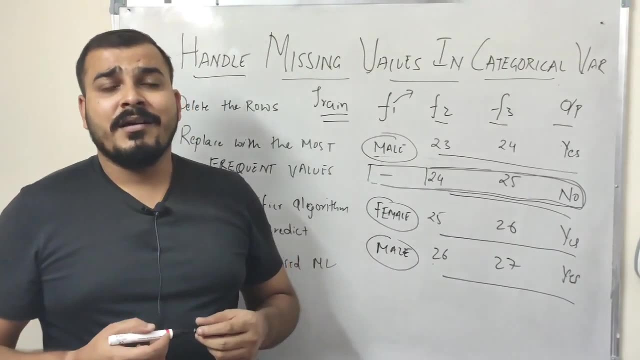 Pretty much simple. I am basically creating a classifier algorithm to find out the missing values in this category feature, And you can apply any classifier algorithm. Let it be k-near, Let it be nearest neighbor, Okay, Different kinds of algorithms. basically, you can basically apply. 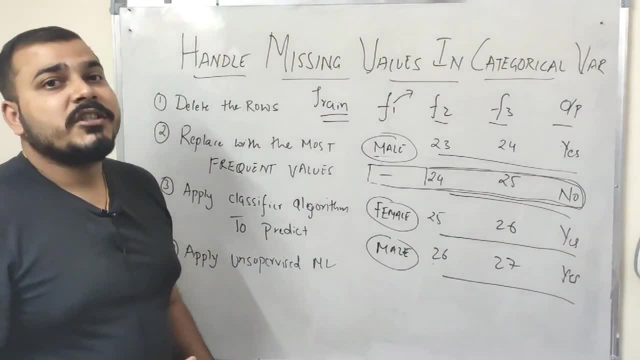 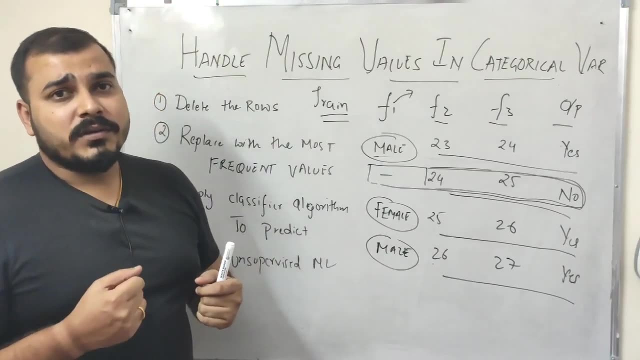 Okay, The last technique is basically: you can also apply an unsupervised machine learning technique. That is basically called as clustering technique. Now, if I take k means clustering, or hierarchical mean clustering. What I will do is that I will skip this column completely. 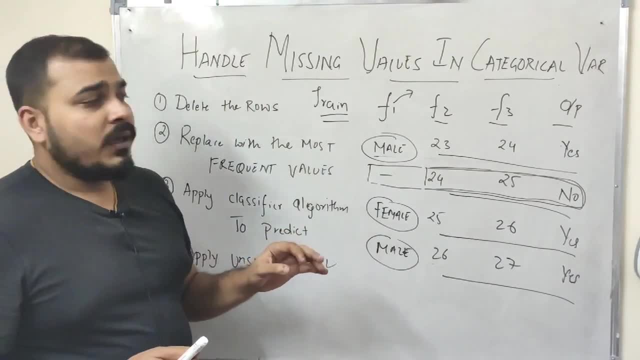 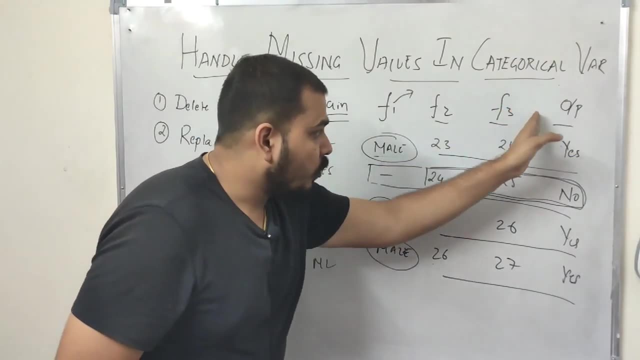 I will skip F1 column. I will skip F1 column. I will take all these values. I will take all these values- F2,, F3 and output Okay, And don't require output also. Okay, Let me just cancel out output.